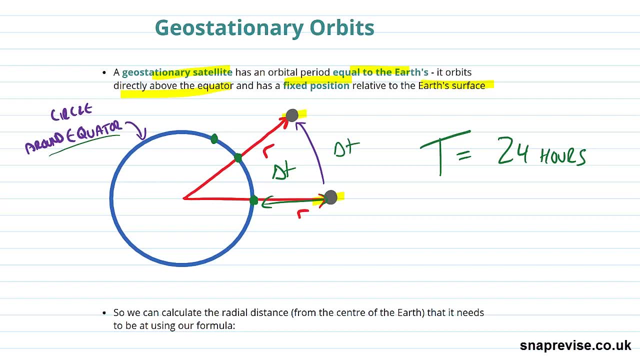 for the Earth and Moon. excuse me, it would be like the Moon orbiting around the Earth at exactly the same rate that the Earth turns. So this satellite moves at exactly the same rate, orbiting around the Earth. So a year- what I mean by a year- for this satellite? 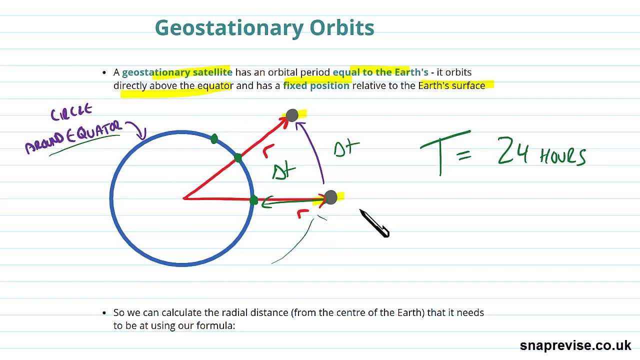 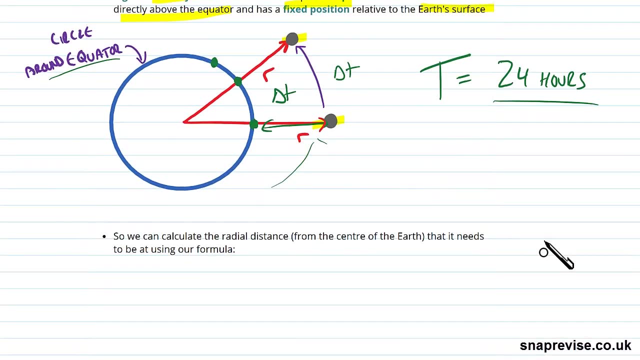 I mean, the time it takes for it to go all the way around and come back is the same as the turning rate of the Earth, the rotational rate of the Earth, And that's the significant thing. So we can actually work out what that has to be because, remember, we have this relation. 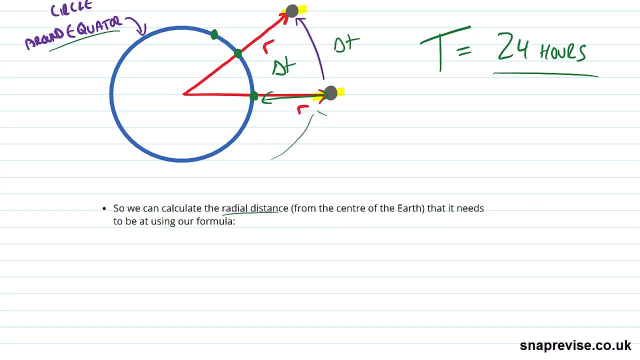 between the period of a satellite and its radius of its orbit. So we can calculate the radial distance from the centre of the Earth that it needs to be at by using our formula that we had before. Remember we have that r cubed over t squared is just equal. 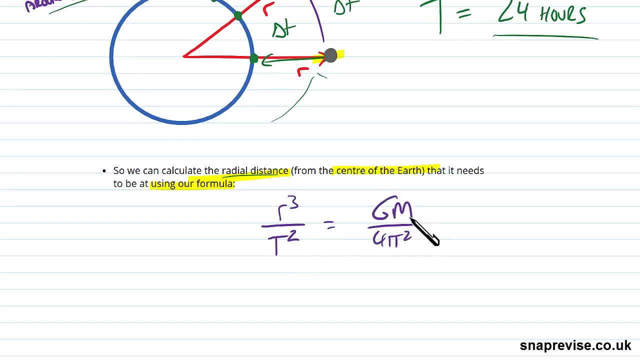 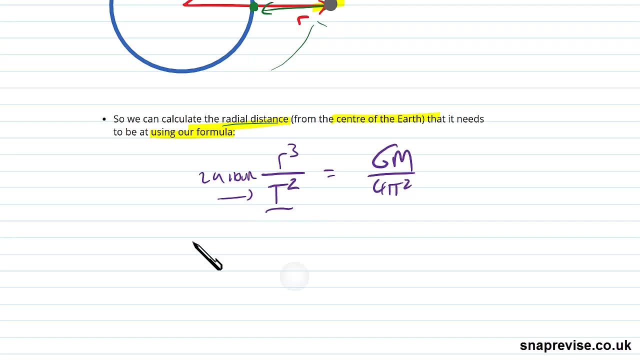 to gm over 4 pi squared, where m is the mass of our object. So now we know what t is. t is 24 hours, So we can basically find that r cubed is just going to be equal to g times m times t squared, all divided by 4 pi squared. Now what is t? We know that t is 24 hours. 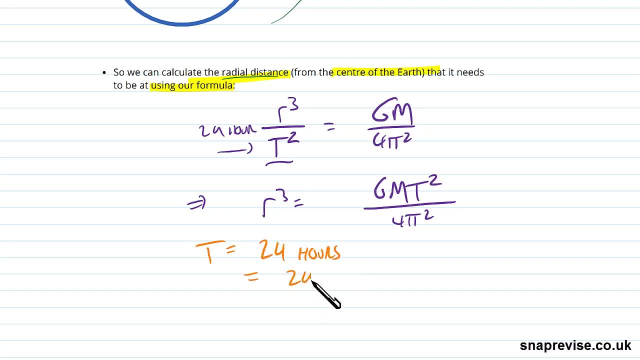 but we need that in seconds. So t is going to be 24 times 60 minutes in an hour, times 60 seconds in a minute, And we know that g is 6.67 times 10 to the minus 11, Newton's. 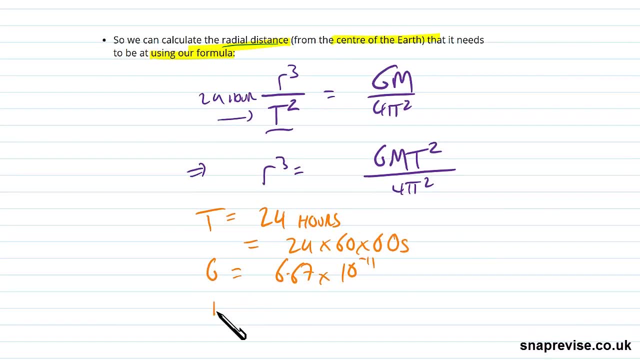 gravitational times, the universal gravitational constant. We know that the mass of Earth is here. we'll take it as 6.0 times 10 to the 24 kilograms. Hey guys, to continue watching this video and unlock hundreds of other super concise. 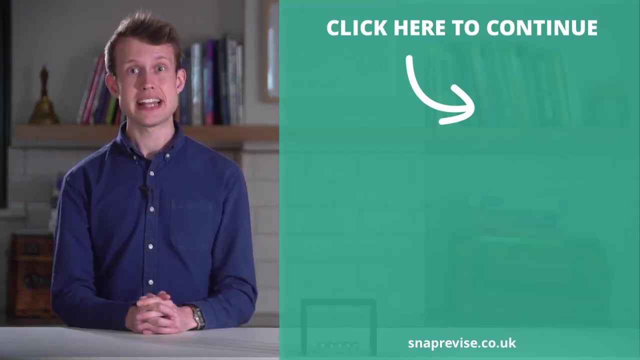 and exam board. specific A-level physics videos: just click the Snap. Revise smiley face. Join me today and together let's make A-level physics a walk in the park.